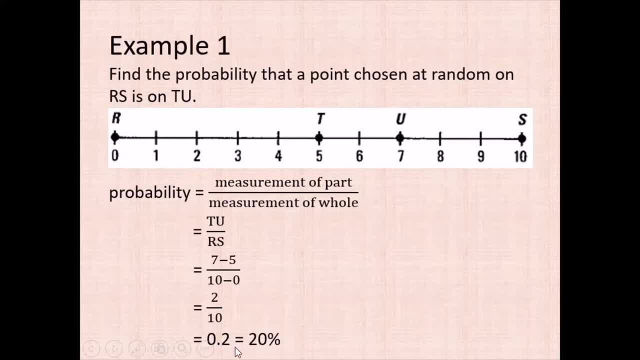 And the percentage you can either times by 100, because it's per cent, and that's what cents means- 100, so it's literally per 100. You'll get 20. Or you can move the decimal over two places. It's kind of the shortcut here, So you'd have to add a 0, move it over two places. 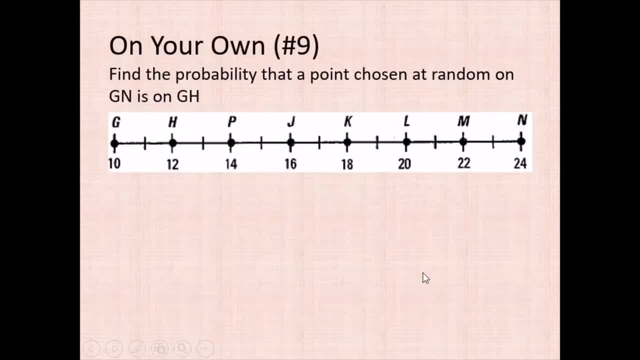 and it'll be 20%. All right, you guys can try this one. So pause the video, try it out. The answer is a decimal, so it won't be a nice 20% like in example one. So if you're wondering, 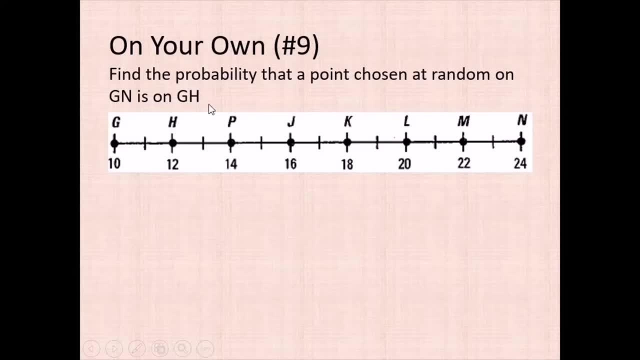 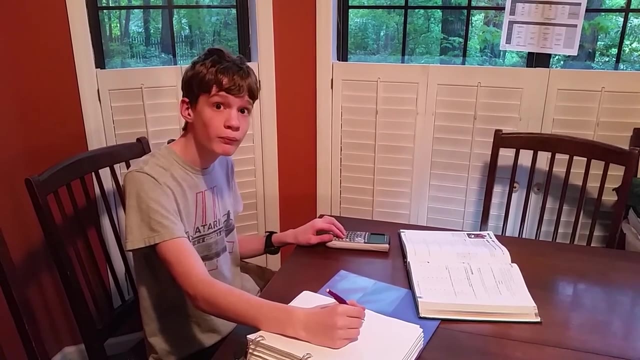 about that. you're on the right track And we're doing GN on GH, So go ahead, pause the video and, once you've got it, resume it and we'll see if you're right. Hey, Caleb, Yeah, Last night I had this dream and I was swimming in orange soda. 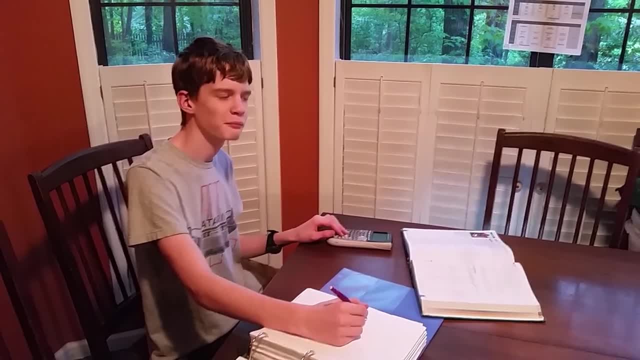 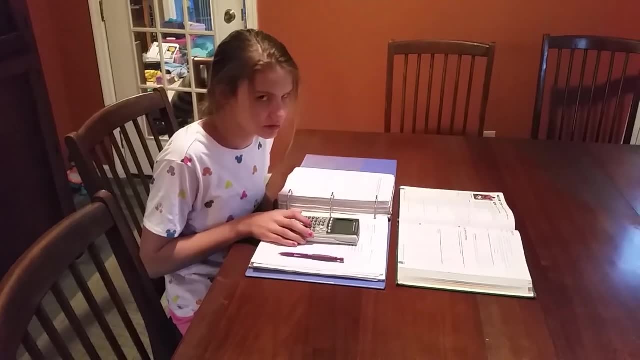 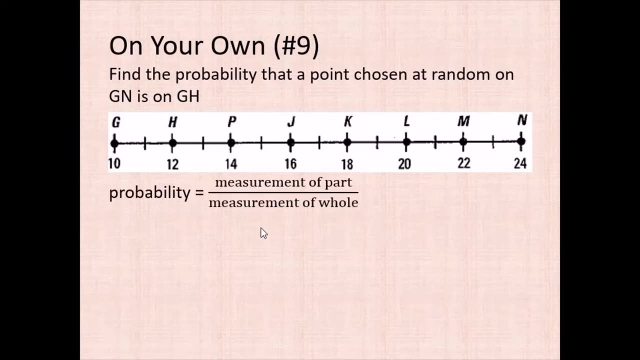 You did. Yeah, it was a Fanta C. Okay, Okay, Okay, Okay, Okay Okay. The calculator isn't working. Why Is it unemployed? Okay, so our probability is the measurement of the part, and the part is the GH. 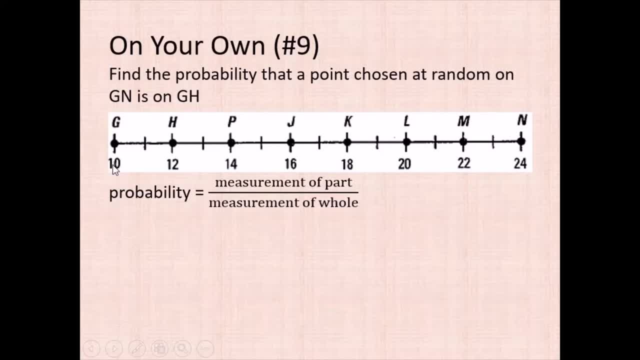 It's a little tricky because it starts at 10.. Hopefully you noticed that and didn't think that was a 0. But it's 12 minus 10 for the GH part and that's 2.. So 2 is going to be on the top. 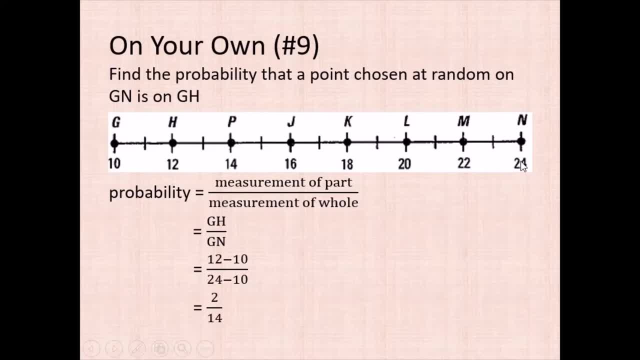 And then the whole thing is It's not 24, but it's 24 minus 10.. So make sure you have that. You subtract the 10 and didn't think it was a 0. And that would be 14. So it would be 2 over 14.. Divide that out and it's 0.14, with some more decimals. 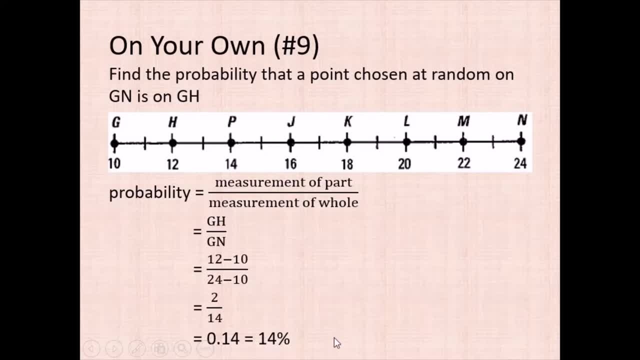 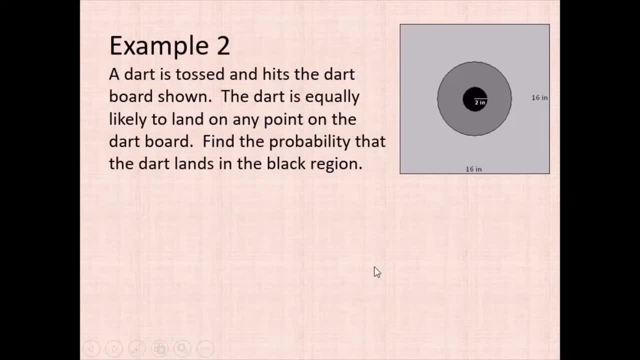 And it comes out to. You can round it to 14%. I think it's 14.3% if you had more decimals than that. Okay, let's look at our last example. here We've got a dart board. A dart is tossed and hits the dart board as shown. 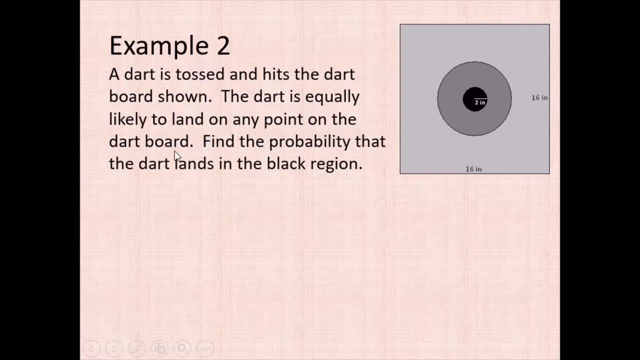 The dart is equally likely to land on any point on the dartboard. Find the probability that the dart lands in the black region. Okay, so obviously this person can't aim, which is why it says it's equally likely to land on any point on the dartboard. 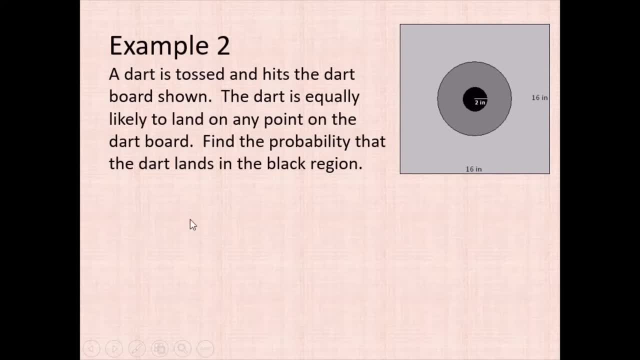 Like least they can hit the board, I guess. Anyways, skill aside, let's look at this. Um so Yes, region is a circle with the radius of 2 inches, So we're going to use our circle formula, which is pi r squared, and put 2 in for that, pi 2 squared and whatever. 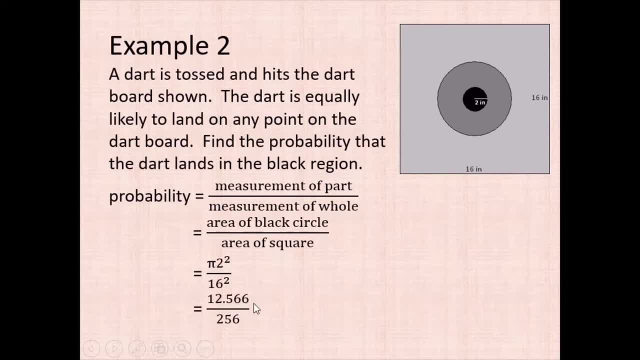 that is apparently that is 12.566.. So that's going to be our top number. The measurement of the whole thing would be the whole dartboard in this, this 16 by 16 square, And so we would do 16 times 16 for the bottom, or 16 squared, and that's. 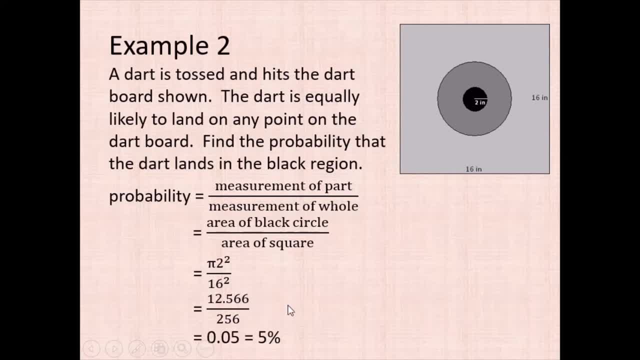 256.. We would divide these two numbers and we get 0.05, and then times it by 100 to get our 5%. So 5% probability of hitting a bullseye. So I guess, if you were just throwing this randomly- 1 out of every 20 or so, because that's 5%- 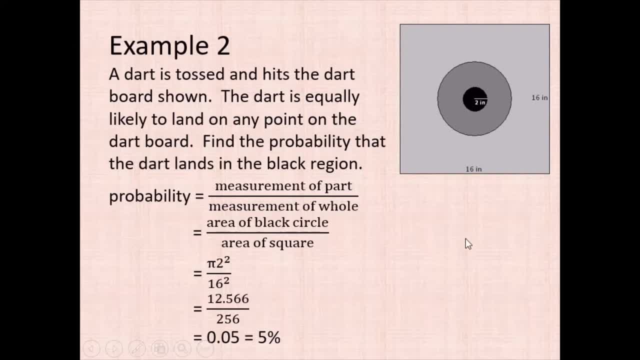 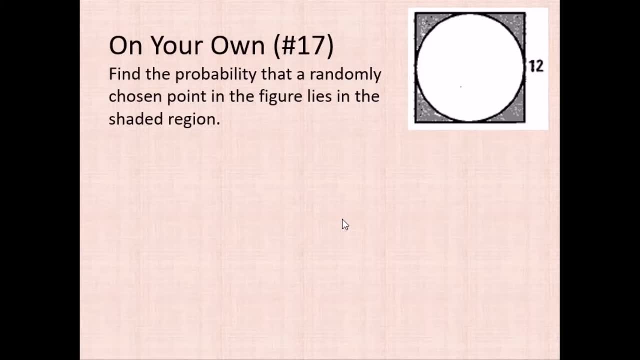 would hit this Interesting. Okay, so you've got an on your own. It says: find the probability that a randomly chosen point in the figure lies in the shaded region. The shaded region is not really like a square or a rectangle or something, But see if you. 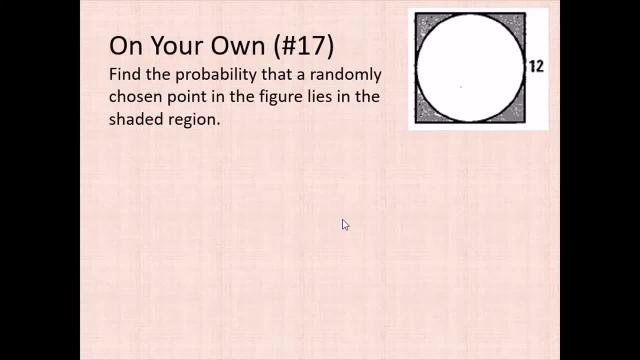 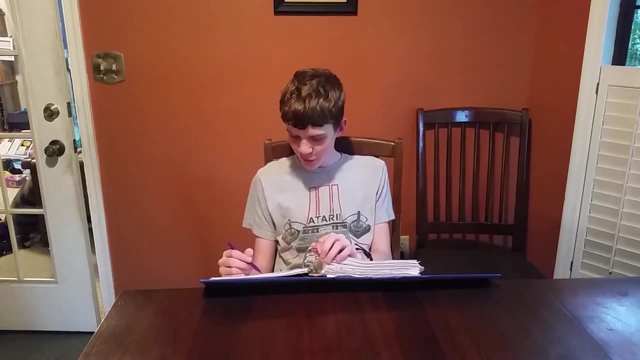 can figure that out. give you a hint: There's a little bit of subtraction going on. Pause the video, see if you can figure out the probability of that and once you've got it, resume it. That's interesting. Here's an article about a coin factory shutting down. 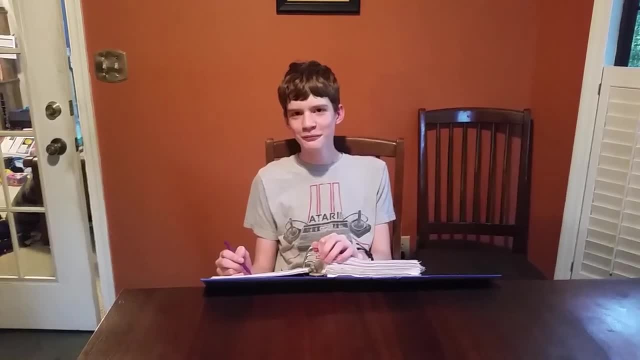 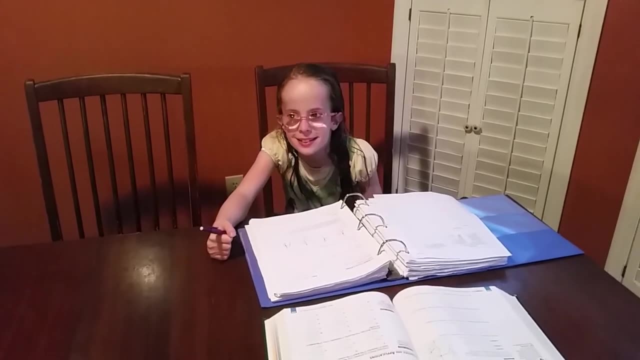 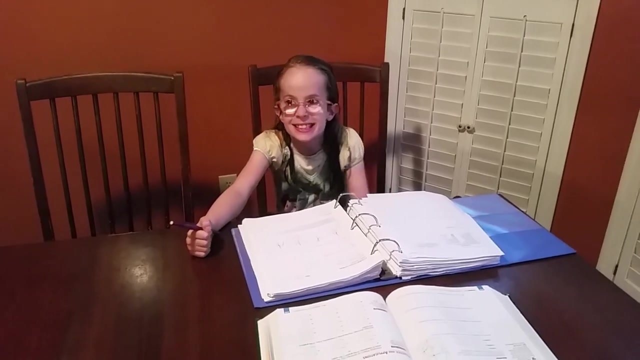 That doesn't make any sense. Hey Sierra, What? What did the janitor say when he jumped out of the closet? I don't know. Supplies, Supplies, Okay. so now we're going to go ahead and see if we can figure out the probability of hitting a bullseye.